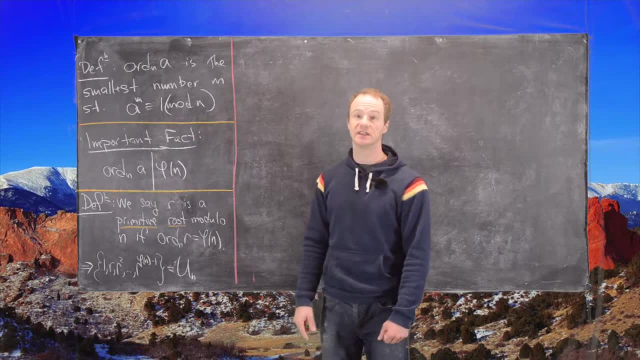 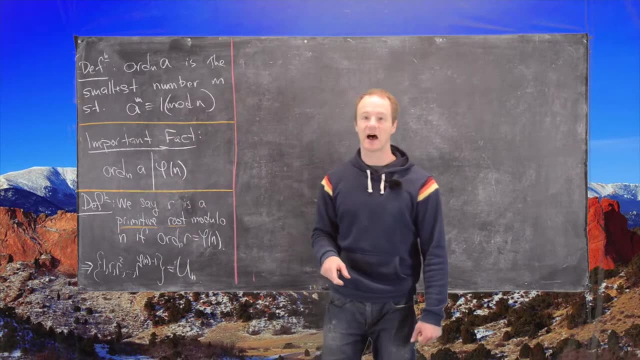 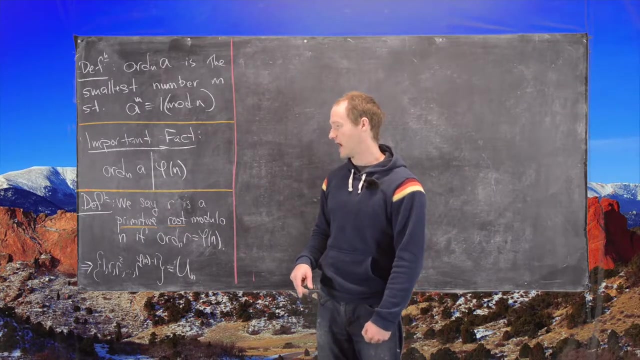 And here we're generally taking the rule that the GCD of a and n is 1.. Then we have this important fact that the order of a modulo n must divide phi of n, which makes phi of n like an upper limit for this order of an element. 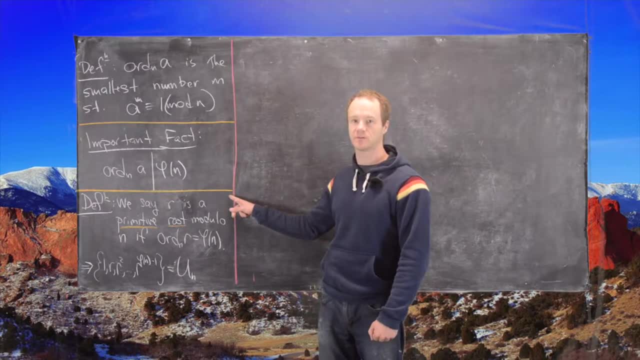 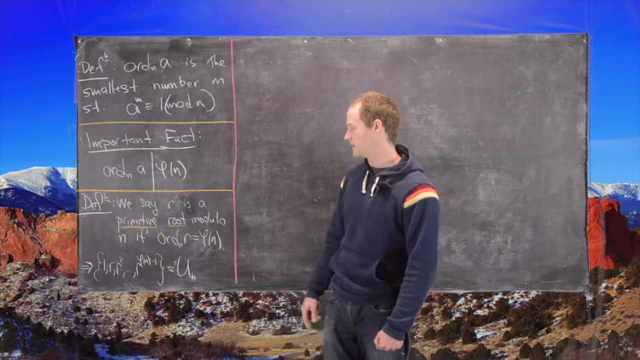 And that upper limit is important. and that brings us to the next definition, which is the following: So we say a number r is a primitive root modulo n if its order modulo n is phi to the n. So if we hit that upper limit, 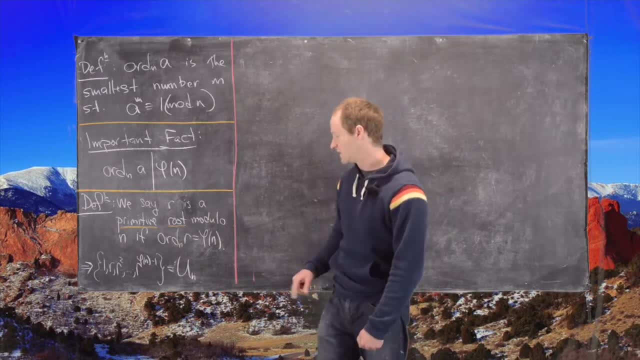 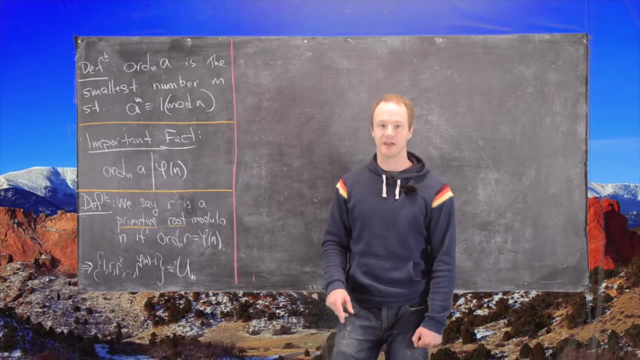 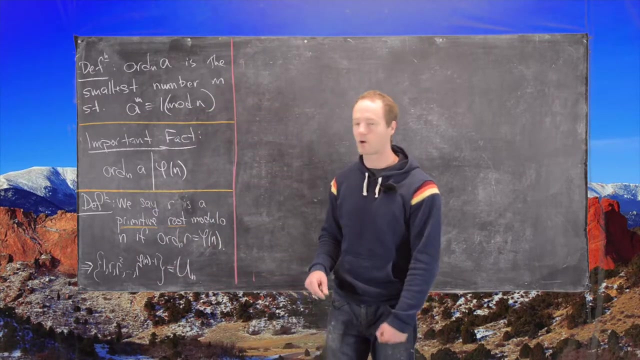 So in terms of the group of units, that means the group of units modulo n, and recall that that is all numbers that are relatively prime to n, between 1 and n. So every number in this group of units can be written as a power of r. 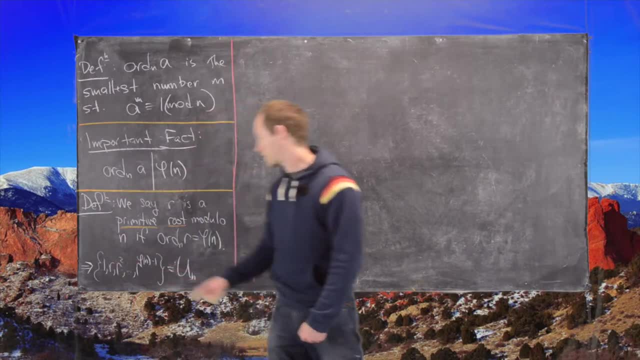 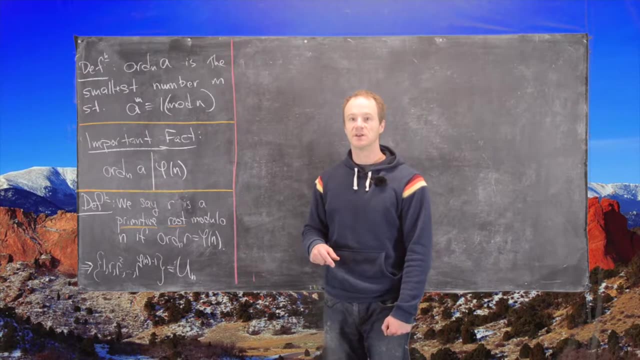 So we have 1, which is r to the 0, r, r squared up to r to the phi of n minus 1.. We don't need to include r to the phi of n, because that itself is 1.. So let's look at some examples of finding primitive roots. 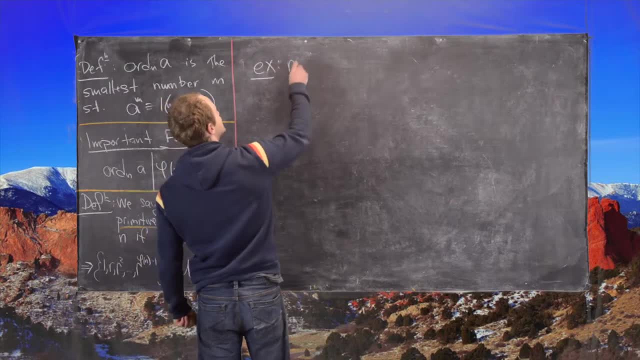 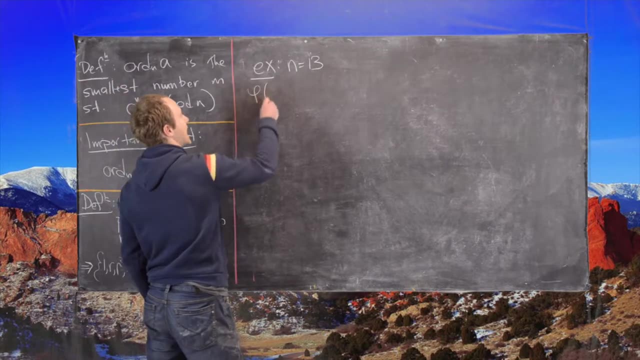 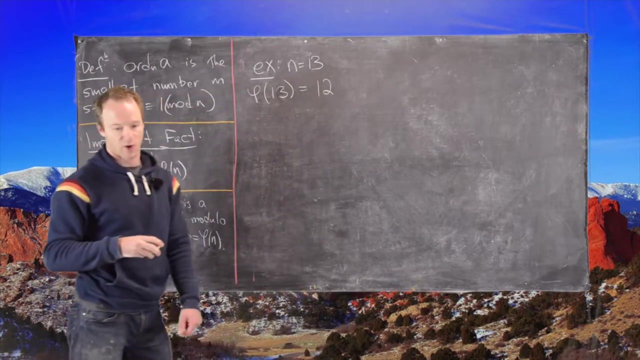 So let's first look at: n equals 13.. So we want to first look at phi of 13, which equals 13 minus 1, which is 12, because 13 is prime, And so that tells us that the possible orders 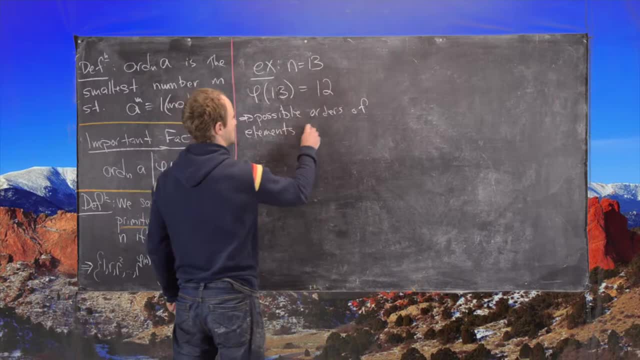 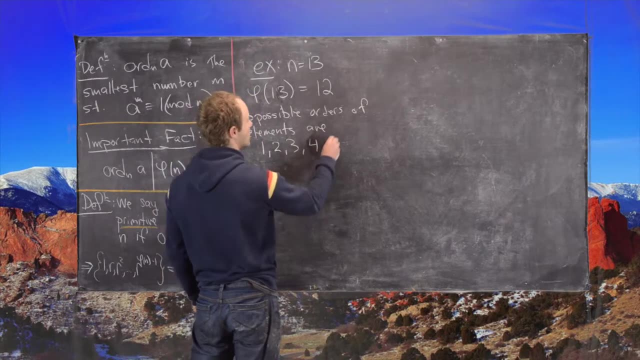 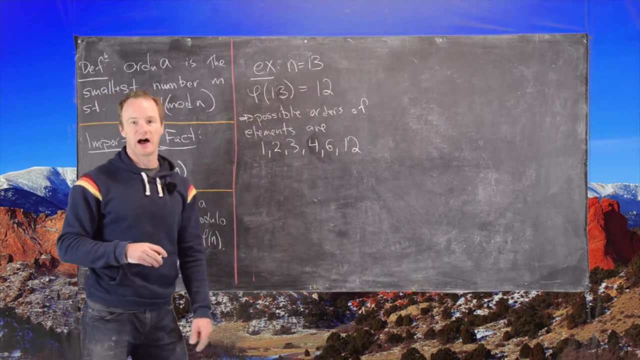 Of elements are 1,, 2,, 3,, 6,. sorry, 1,, 2,, 3,, 4,, 6, and 12.. So, and that's because we know the possible orders must divide 12, and these are all the divisors of 12.. 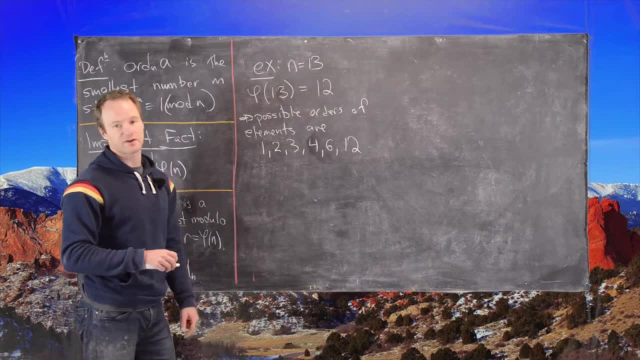 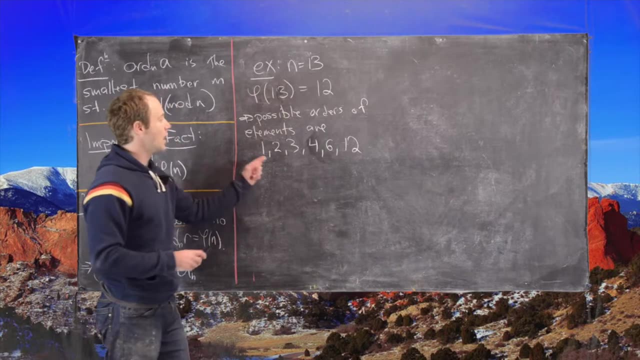 So now what we want to do is pick a number between 1 and 13 and check all of these exponents until we get an exponent that brings us back to 1.. Okay, So 1 will obviously not work, because 1 to the 1 is 1.. 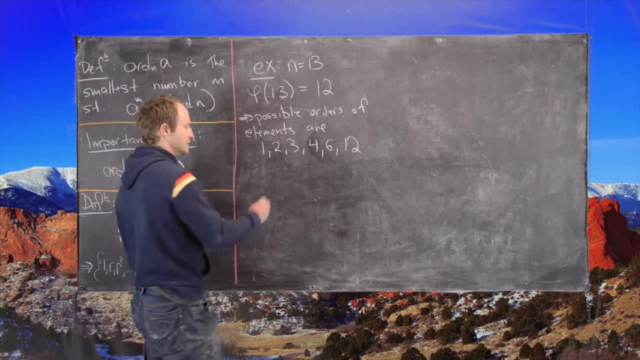 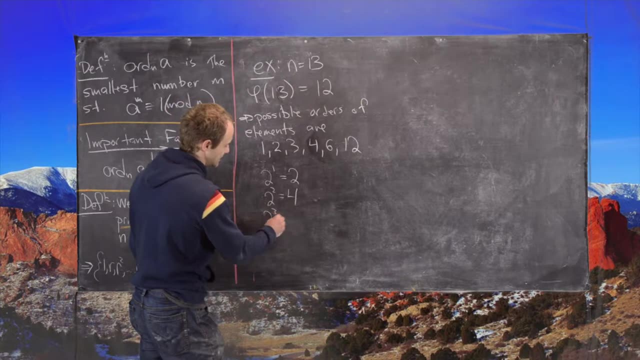 The order of 1 is 1.. So we'll start with 2.. So 2 to the 1 is equal to 2.. 2 squared is equal to 4.. 2 cubed is equal to 8.. 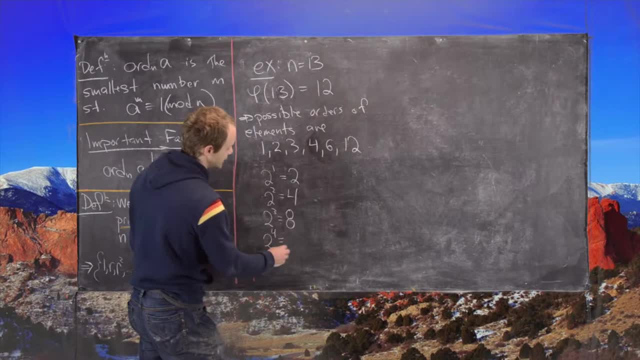 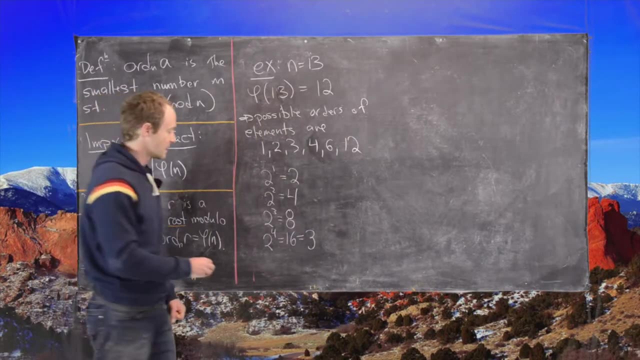 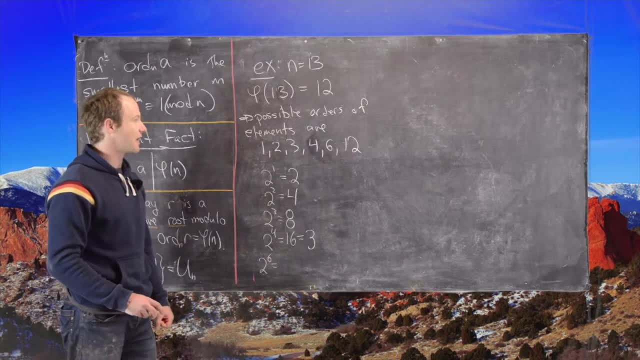 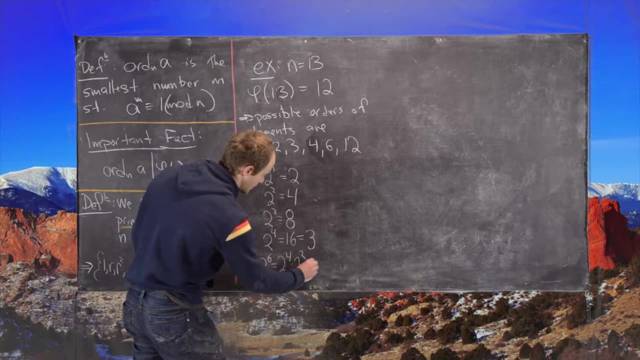 I'll use what's in the back of my list to help me here. So 2 to the 6th is 2 to the 4th times 2 squared, which is 3 times 4, which is 12, which is negative 1.. 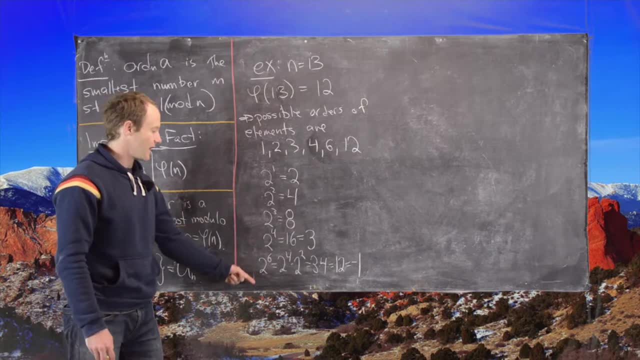 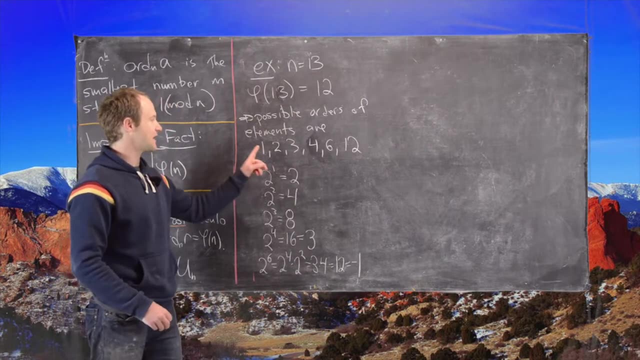 So now, what we notice here is nowhere on this list is 1.. So that means the order of 2 cannot be 1, 2,, 3,, 4, 6. So that means the order has to be 12.. 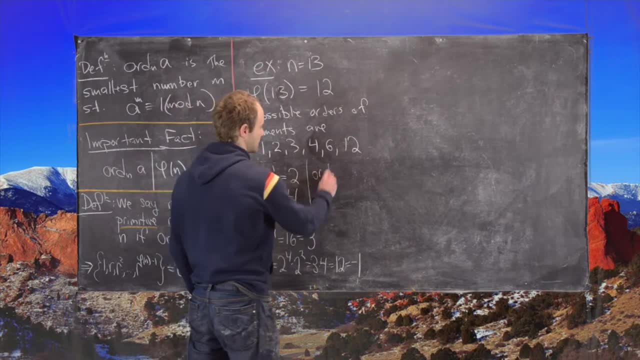 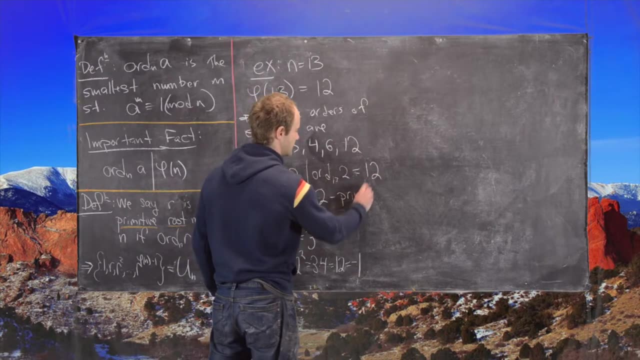 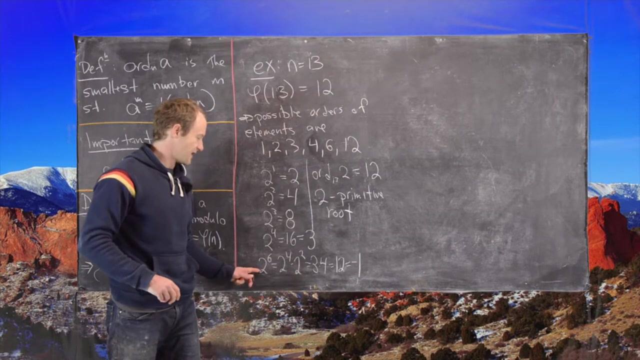 So what we've just shown is that the order mod 13 of 2 must be 12.. In other words, 2 is a primitive root. Now, obviously, at this point it's easy to check that if you square negative 1, you get 1.. 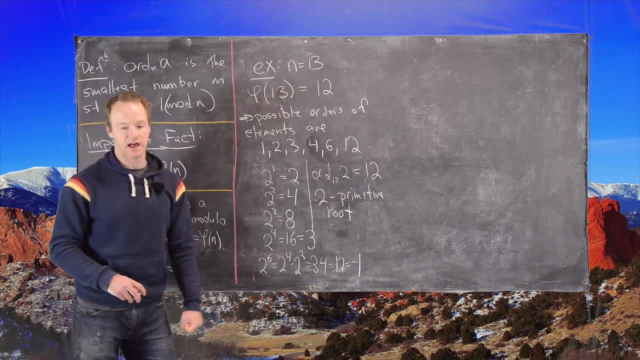 But we don't even really need to do that, because we know that all that's left as a possibility for the order is 2.. So that means that the order is 2, 2,, 3,, 4,, 6,, 7,, 8,, 9,, 10,, 11,, 12,, in other words, phi of 13.. 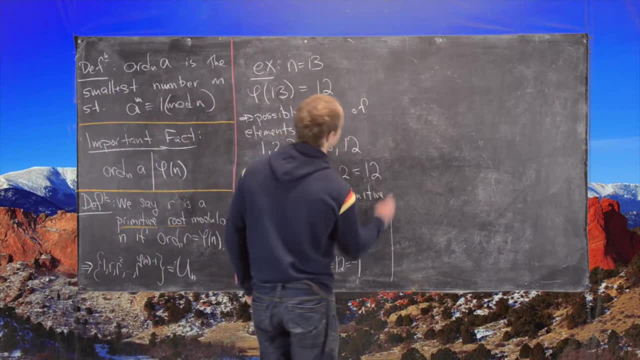 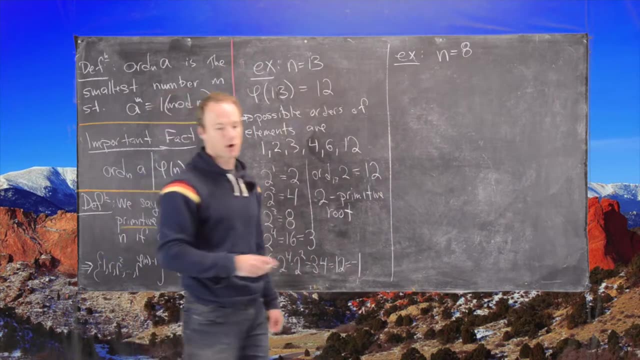 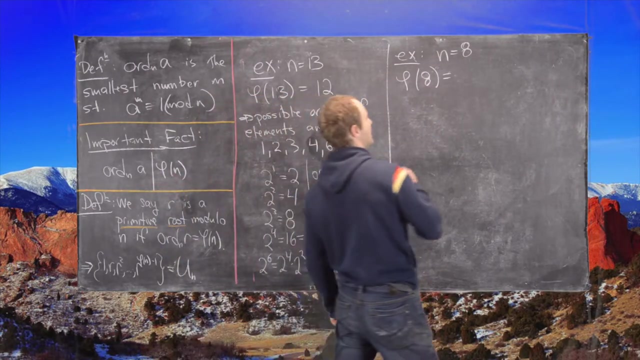 Okay, good, Let's do another example. So let's do: n equals 8. And so we need to calculate phi of 8.. So let's recall that phi of 8 is equal to 8 minus 4.. 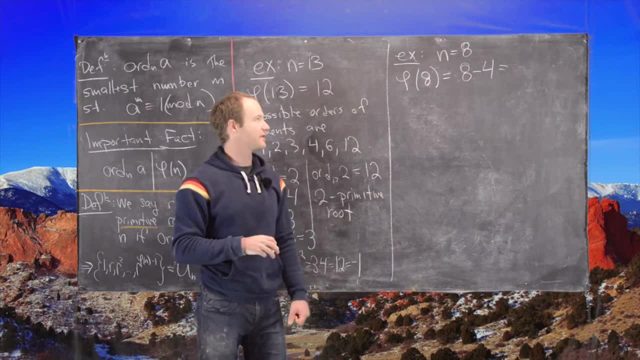 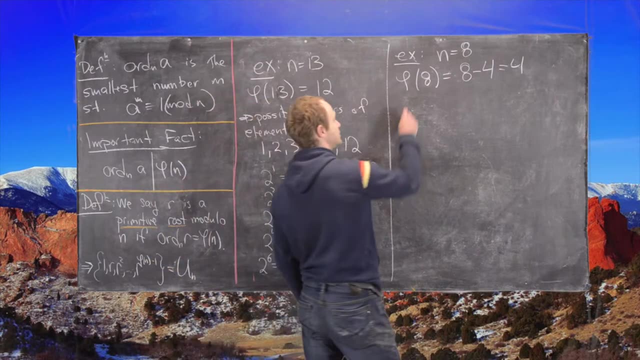 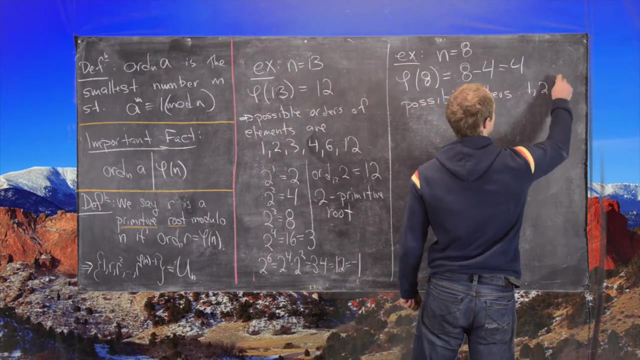 In other words, 2 cubed minus 2 squared, We're using the formula for phi of a power, of a prime, And that is equal to 4.. Great, So that tells us the possible orders are 1,, 2, and 4, because they have to be divisors of 4..